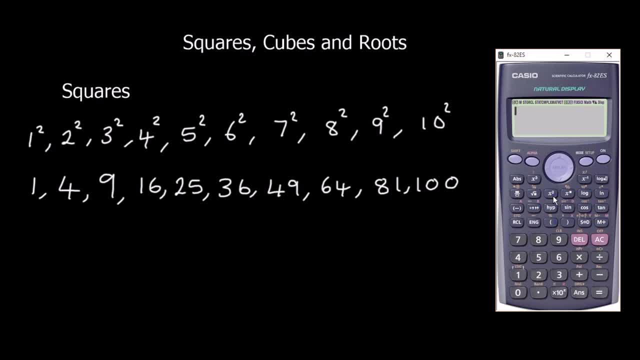 So if you look here on the calculator, there's a squared button. so if we wanted to work out what 12 squared was, we'd type 12, press the squared button, 12 squared. So 12 squared equals 144.. 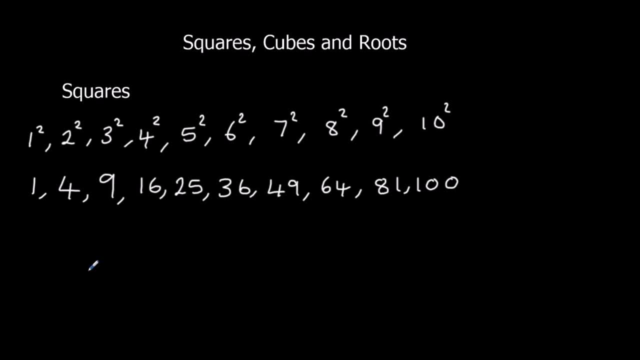 Now what we've got to be careful of, especially when using the calculator, is something like minus 2 squared, Minus 2 times minus 2, minus 2 times minus 2.. So whenever you've got a negative times a negative, it makes a positive. 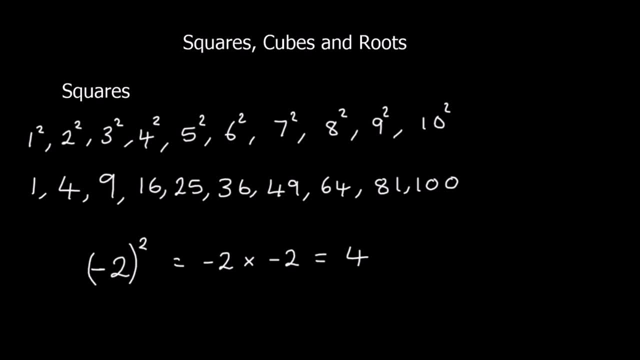 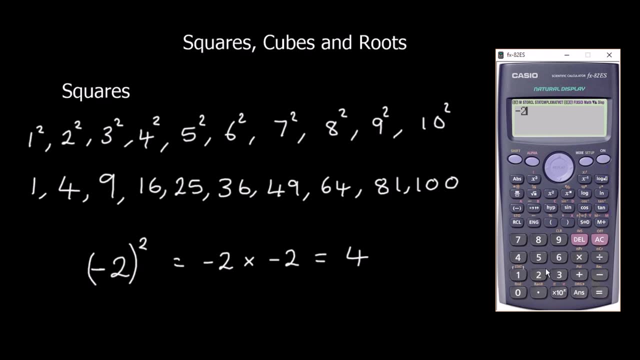 So minus 2 times minus 2. That gives us positive 4.. On the calculator, if you type minus 2 squared, it gives you an answer of minus 4.. That's because it thinks you mean take away 2 squared. 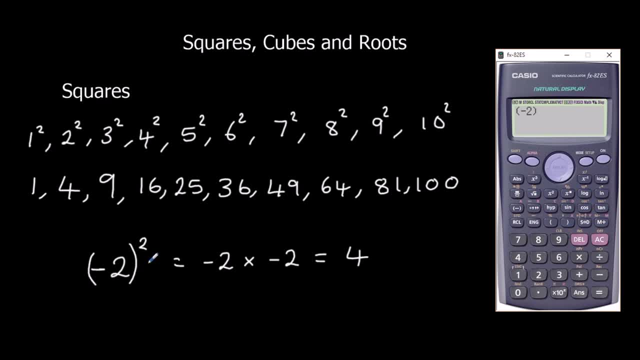 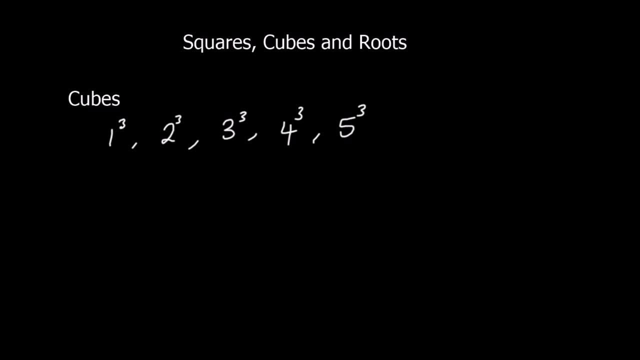 So what you've actually got to do is write the minus 2 in brackets, then press squared and that gives you the answer of 4.. So that's it. So when we've got a cube, it's like a square. 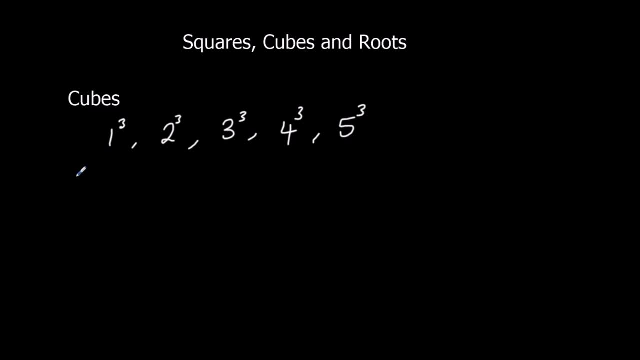 So where a square is times by itself, a cube is times by itself, and then again. So 1 cubed means 1 times 1 times 1.. So that's 1.. 2 cubed 2 times 2 times 2.. 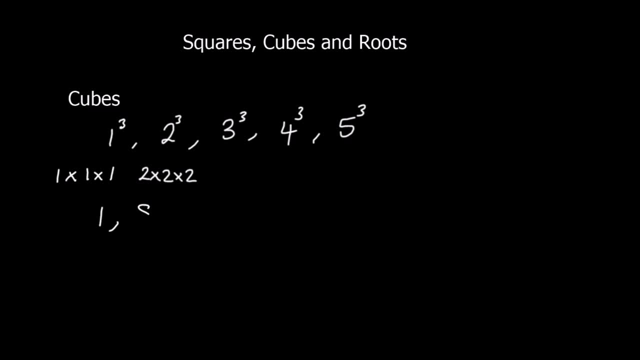 2 times 2 is 4.. 4 times 2. 8.. 3 times 3 times 3.. 3 times 3 is 9.. And then 9 times 3 is 27.. 4 times 4 is 16.. 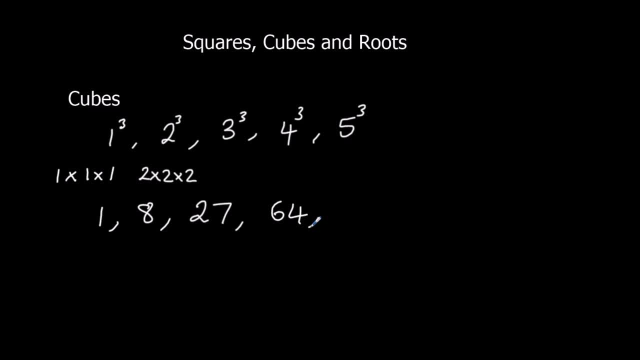 16 times 4 is 64. And 5 times 5 is 25.. And 25 times 5 is 125.. You should know these first 5 cube numbers. Ok, so the opposite of squaring or cubing is rooting.